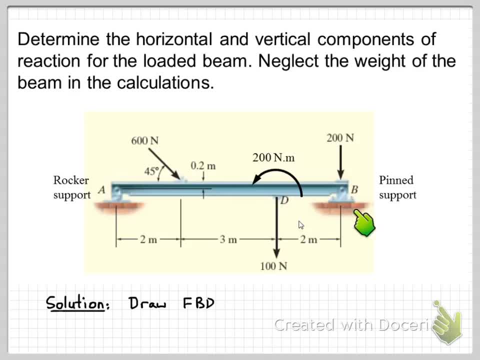 So the things that we'll need to remove are the supports at ends B and at end A here and replace those supports by the forces and or moments that they provide to the beam in order to balance these applied loads. And once we've done that, 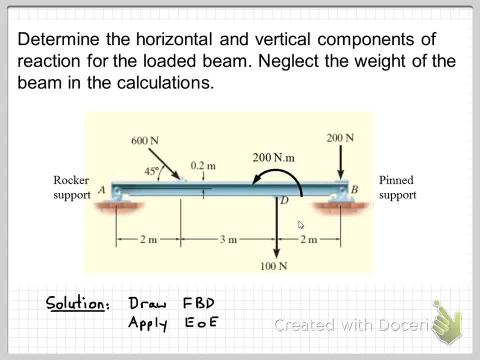 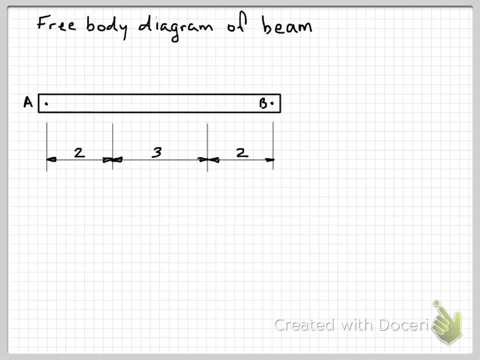 We will apply the equations of equilibrium and then solve the equations of equilibrium for our unknown reaction forces and moments. OK, So let's start by drawing the free body diagram. So our free body diagram, to start with, is just a simple representation of the external. 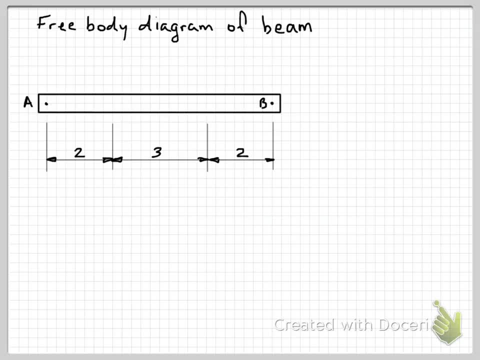 shape of the body that we're analysing. So in this case it's just a simple long rectangle. Yeah, OK, on here the relevant dimensions that we'll need and then, once we've done that, we can start adding in our forces or our loads that are acting on the beam. So in 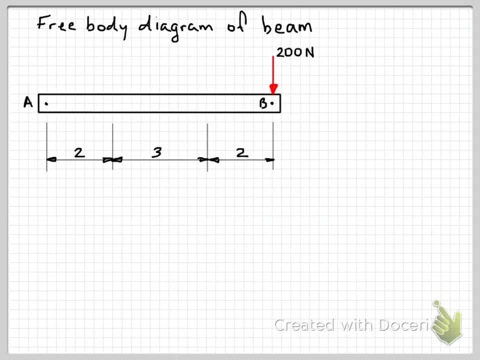 this problem. we'll start from NB and start working our way across. so we've got the 200 Newton force acting downwards at point B and a 100 Newton force acting 2 meters from NB, and there's also a couple moment applied there a few hundred Newton meters and we've got the force 2 meters from NA. 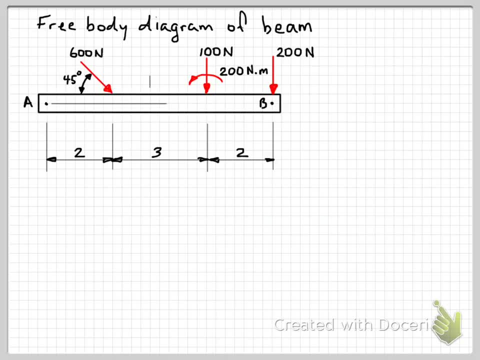 which is 600 Newtons at 45 degrees. and we also take note here that we've given that we've been given the distance between where that load is applied and the center line of the beam. so we've included that dimension in our free body diagram because that will be important for when we're calculating moments. 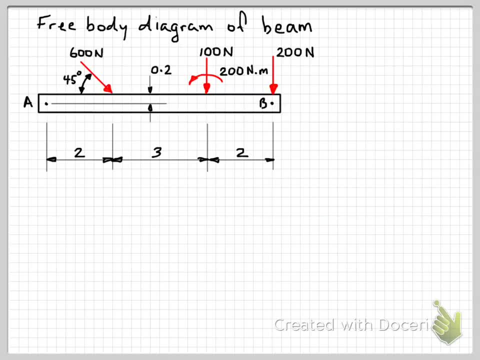 Okay so. So now that we have all our loads indicated on our free body diagram, we can start thinking about the reaction forces. So at end B here we have a pin support, so rotation is allowed. so there's going to be no moment reaction, but the beam is constrained from moving horizontally and also constrained. 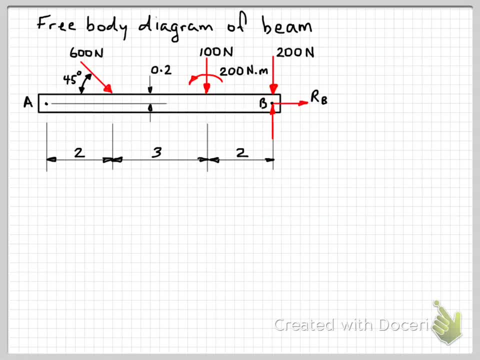 from moving vertically. so we're going to have a vertical reaction force and a horizontal reaction force at point B and we label them with appropriate variable names. So we'll have R, subscript B, subscript X for the reaction force at B in the X direction, and similarly for the vertical reaction force, R for the force, B for where it's acting, and 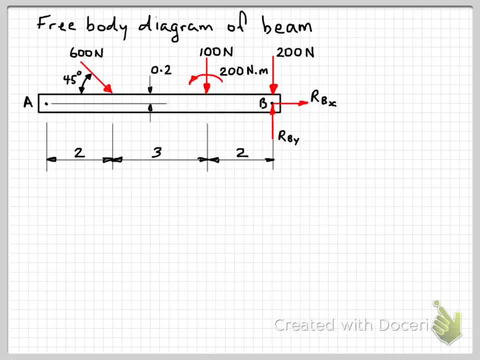 Y for the direction. Then at end A we have a rocker Support, so it prevents translation in the vertical direction but allows some movement in the horizontal direction. so we'll have here just a single vertical reaction RAY. Okay, so now that we have our free body diagram and our unknowns identified and labelled, we 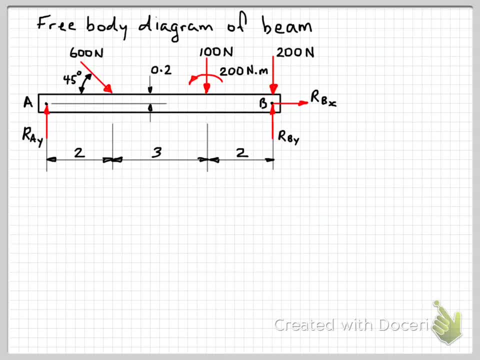 can start to write out the equations of equilibrium to solve for those unknown reaction forces. Okay, so we've got three equations of equilibrium, some of the moments and two force component equations. Which one do we start with first? well, usually we start with the moment equation because 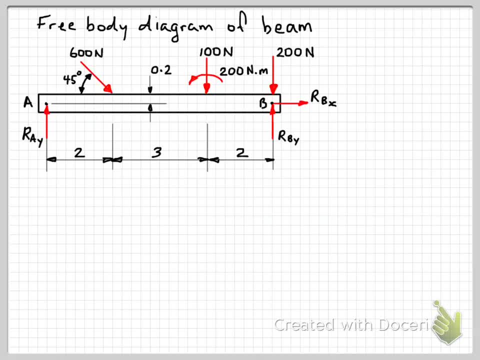 that enables us to usually take out one or more of our unknown reaction forces so that we end up with just one equation and one unknown, so that we can solve for that one unknown straight away. So in this problem we could take moments about point A, as that would take out the effect of RAY as moment of RAY about point A would. 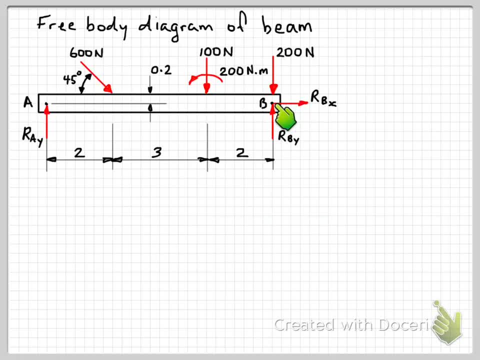 be zero. But we also notice that RBX also passes through point A, so that also will have a zero moment about point A. So in this case we could take moments about A or B, and in either case we'd only have one unknown in the equation. So if we take moments about 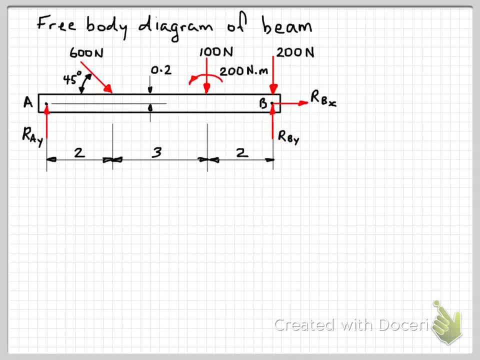 point A, the only unknown will be RBY, and if we take moments about B, the only unknown will be RAY. So in this problem I'm going to use moments about A and again it's important that we indicate in our writing of the equation of equilibrium where we're taking moments. 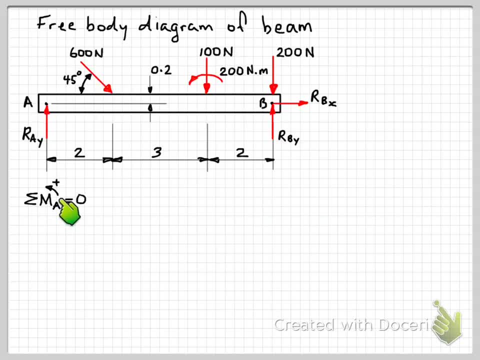 about. So here I've said some of the moments about point A and I also indicate that anticlockwise is positive. So we're just going to work our way from left to right along the beam, taking into account or calculating the moment effect of each of the loads along the beam as we move along. 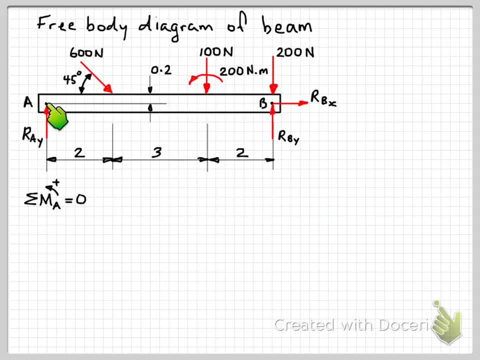 So, starting at point A, as we discussed, RAY has a zero moment about point A because it passes through point A. then we next need to deal with this 600 N force at 45 degrees. So, in my opinion, the easiest way to deal with. 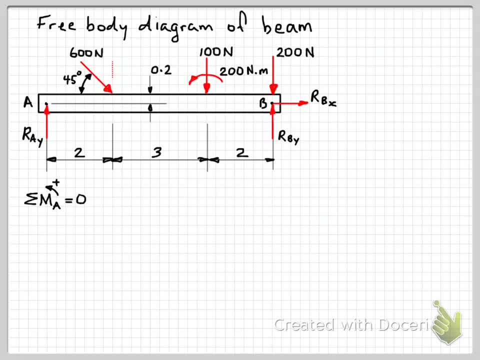 this is to use RAY. The easiest way to do this is to find the horizontal and vertical components. So let's go ahead and do that. So they'll be acting there like that and from trigonometry we know that the vertical component here will be 600 sine 45.. We're given this angle here, 45, and 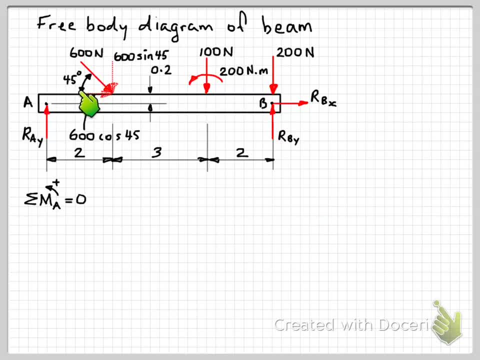 this horizontal component here will be 600 cos 45.. Okay, Let's start with the horizontal. So this is the vertical component of the 600 N force. So its moment effect will be 600 sine 45 times distance, perpendicular distance to point A, which is 2.. So we'll have 600 sine. 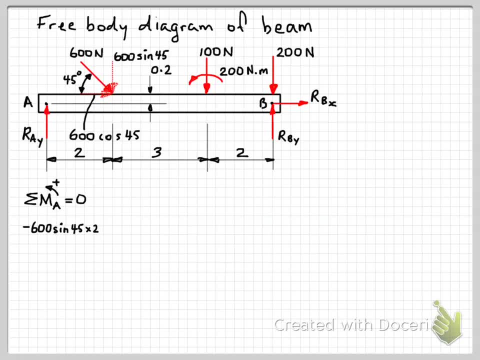 45 times 2, and that's going to be rotating around clockwise, So that's a negative moment according to our positive convention. Before we go on to continue calculating the moments, I just want to point out that I see a lot of people put the component of the force here or up here like this: Draw their components. 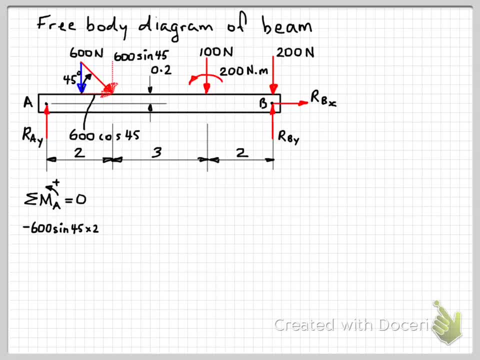 like that. If you do that, in my opinion that's not good practice, because what it indicates is that when you're calculating the moment of this component here, it looks like that the distance between that component and point A is something less than 2.. But the moment. 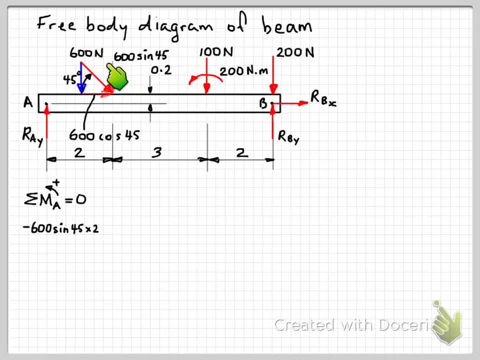 effect of this component is actually the component acting out here times 2.. So try to avoid drawing your components like that. Instead, draw them so that they're in the right place. Okay, Okay, Okay, Okay, Okay. Maintain their correct line of action. 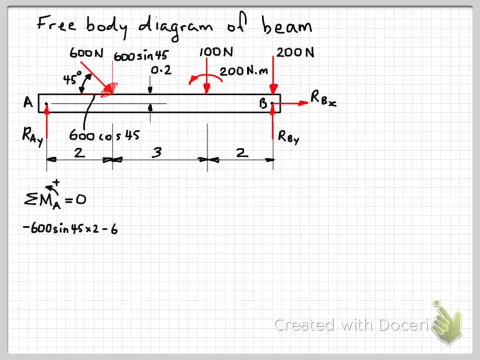 Okay, So next we'll deal with the horizontal component. So again, that's going to cause a clockwise rotation about point A because this force is up here. It's going to cause clockwise rotation about point A. So we have 600 cos, 45 times this distance, which is 0.2.. 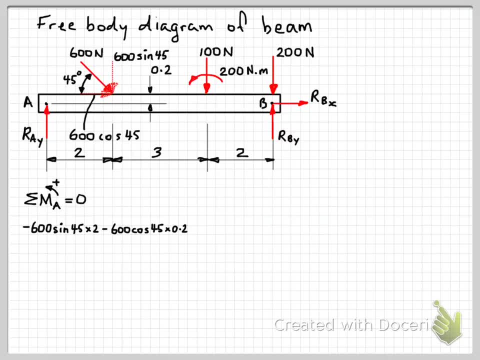 Okay, Alright, then moving along the beam to our 100N force, again, that's going to generate a clockwise rotation- or tend to produce a clockwise rotation- of the beam about point A, and its distance from point A is 5, so its moment effect is minus 100 times 5.. 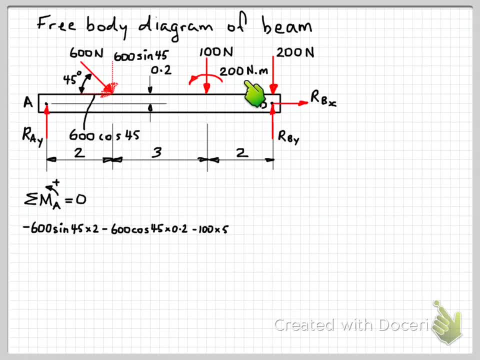 Okay, then we have the 200Nm applied couple moment, so we can just add that in. so plus 200Nm. Now be careful here. in this case our dimensions are in metres and our forces are in newtons, so sometimes you'll have newtons and millimetres as your dimensions. and if you've got a moment, 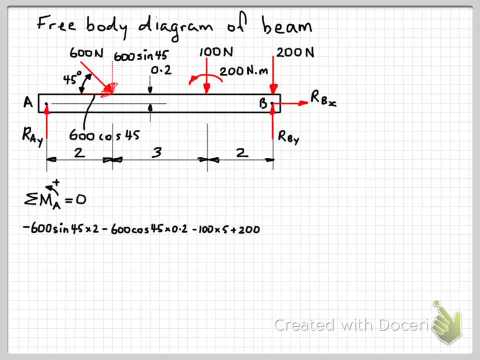 specified in newton metres, then you'll of course need to do the appropriate unit conversion to that, To convert either your dimensions here into millimetres or convert your moment into newton millimetres. Right then, moving along to the end, we've got our 200N applied force here, acting at 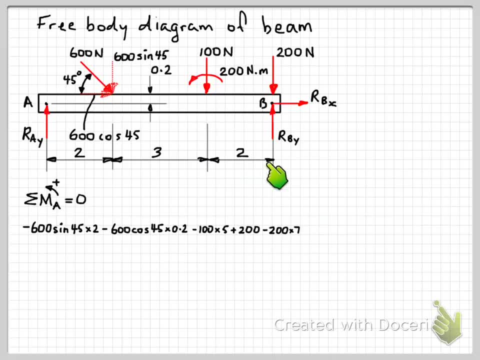 a distance of 7 metres, so the total length of the beam. and again that's causing the clockwise rotation of the beam about point A, so a negative moment. and then, lastly, we have our reaction force, RBY, also acting at 7 metres but causing an anti-clockwise rotation. 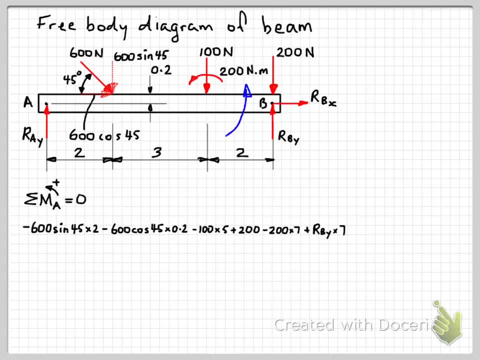 about point A. so that's a positive moment. And all of that is equal to zero. Okay, so that gives us one equation, One unknown in RBY, so we can rearrange that. do the maths to calculate for RBY to get. 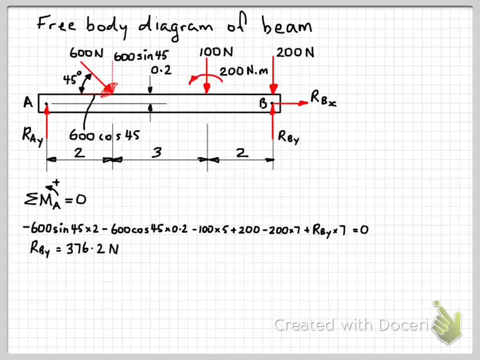 376.2 newtons. Okay, so now we can use our other equations of equilibrium. So, firstly, we'll do some of the forces in the vertical direction, with positive being upwards, all equal to zero. so again, just start by working our way along from left to. 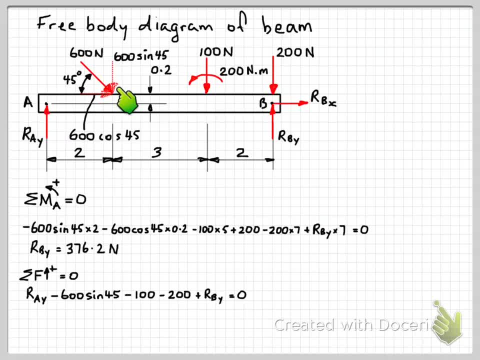 right. so we have RAY positive minus 600, sine 45, minus 100, minus 200, plus RBY, all equal to zero. So we've just calculated RAY up here. so we have again just one equation, one unknown. 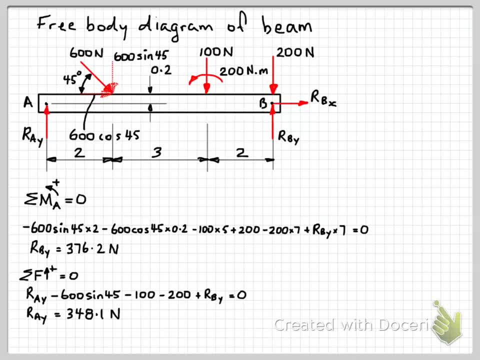 we can solve for RAY. Sorry, I think I just said that wrong. So up here we had RBY that we calculated previously in this equation. RAY is our unknown, so we can substitute that RBY into here and calculate RAY. 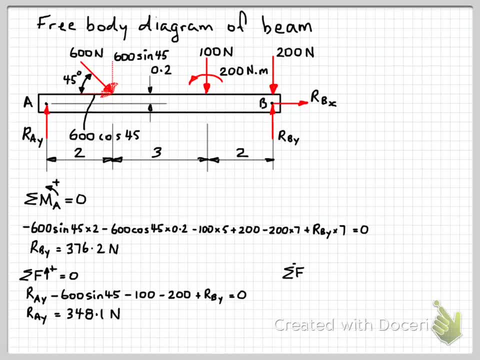 So then we can apply our other equation of equilibrium: sum of the forces in the horizontal direction equals zero to the right being positive. and again we'll just work from home left to right. so we start off with the horizontal component of our 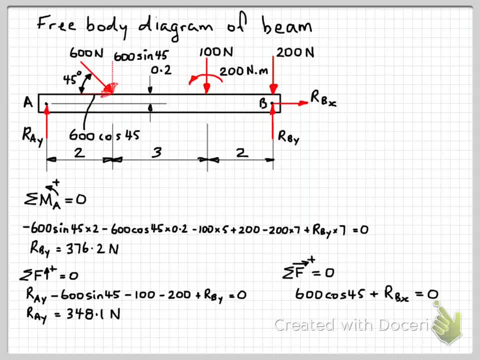 600 Newton force here, so 600 cos 45, and the only other horizontal force that we have is Rbx. so we can solve from that equation to get Rbx equals minus 424.3 Newtons. OK, so now I'll just write out our final answers at the end. 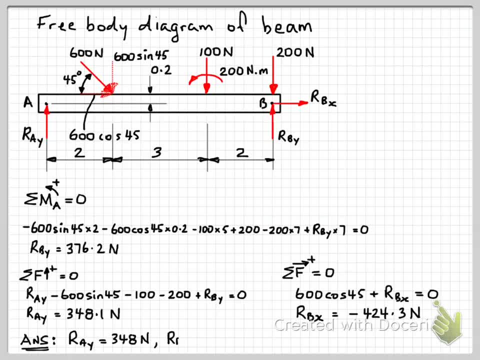 so R A Y and round up to three significant figures. so R A Y is 348 Newtons. Rbx is minus 424 according to what we've put in our free body diagram. so where we had Rbx acting to the right, the negative sign indicates that.